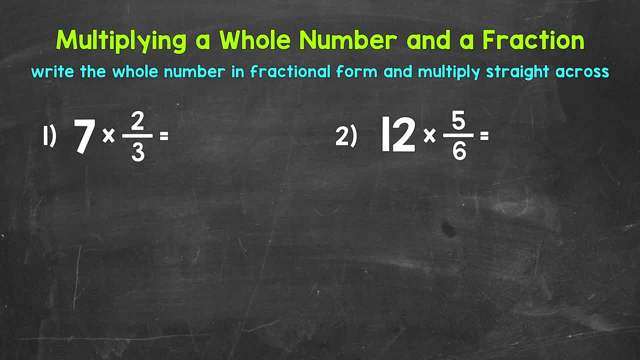 So let's write 7 in fractional form. Now, in order to write a whole number in fractional form, all we need to do is put it over 1.. We're not changing the value of that whole number. We are just again putting it in fractional form. 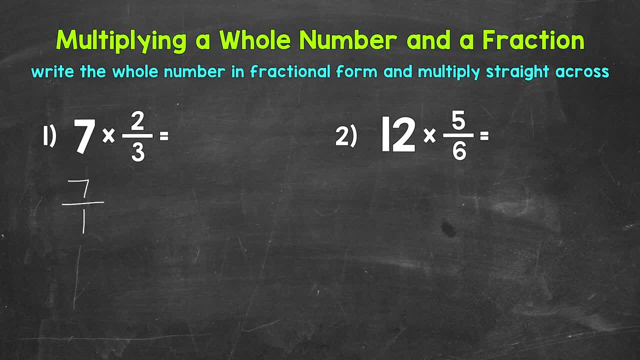 So we're not changing. the value of 7 over 1 still has a value of 7.. Then we have times 2, thirds. Now we can multiply straight across. Let's start with the numerators. So the top numbers 7 times 2 is 14.. 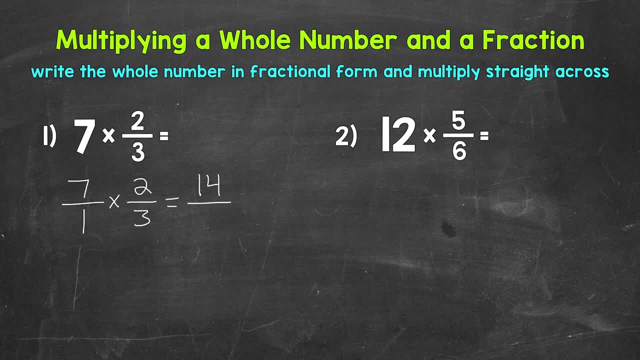 Now for the denominators, the bottom numbers: 1 times 3 is 3.. So we get 14 over 3.. 14 thirds. Now that is our answer, but it is an improper fraction, So let's convert it to a mixed number. 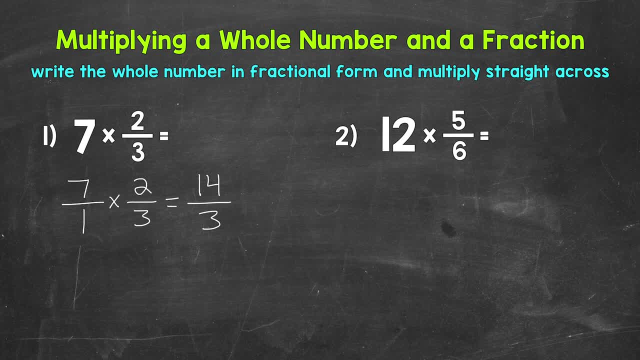 We do that by dividing the numerator by the denominator. So 14 divided by 3. How many whole groups of 3 in 14?? Well, 4.. That's the whole number, part of our mixed number. Now we don't hit 14 exactly. 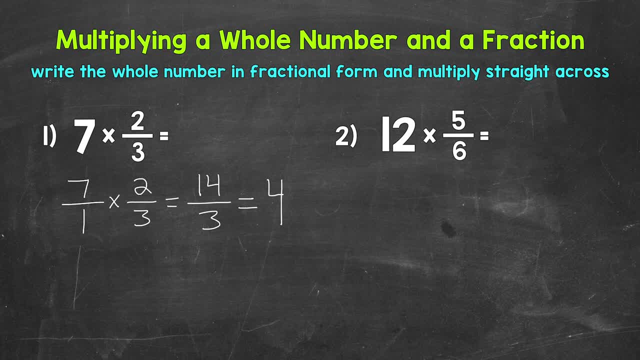 4 whole groups of 3 gets us to 12. So we have a remainder of 2. That way we have a whole group of 3.. That remainder is the numerator of the fractional part of the mixed number. And then we keep the denominator of 3 the same. 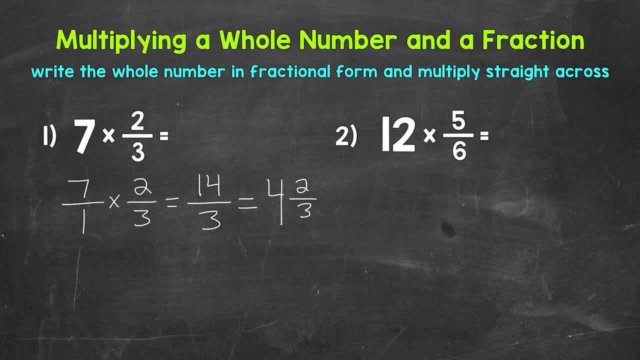 Always look to see if you can simplify the fractional part of a mixed number. 2 thirds is in simplest form: The only common factor between 2 and 3 is 1.. So we are done. Final answer: 4 and 2 thirds. 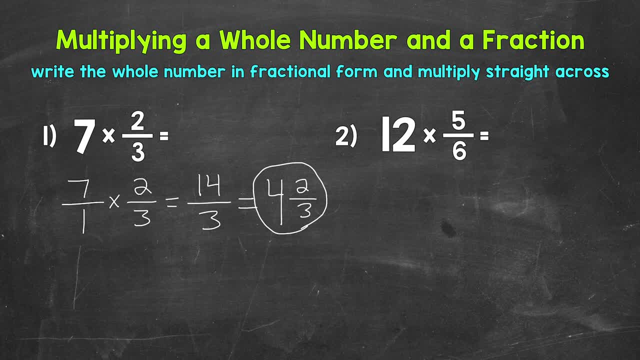 Now, just as a quick recap, as far as how we went from 14 thirds, 14 over 3, that improper fraction to the mixed number. again, we divided the numerator, so 14, and we divided by the denominator 3.. 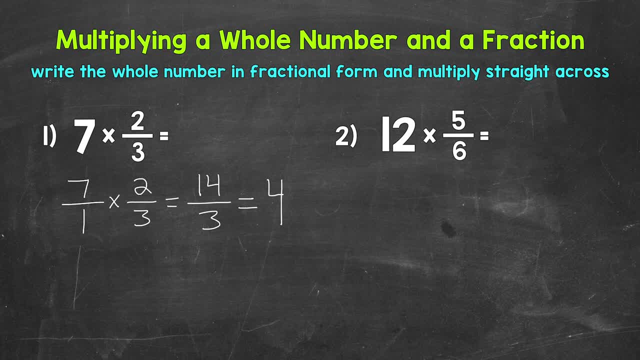 4 whole groups of 3 gets us to 12. So we have a remainder of 2. That way we have a whole group of 3.. That remainder is the numerator of the fractional part of the mixed number. And then we keep the denominator of 3 the same. 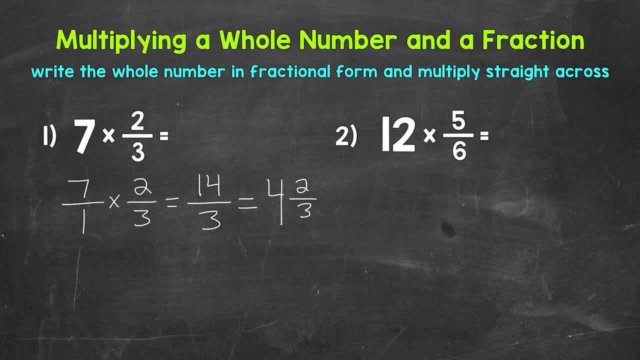 Always look to see if you can simplify the fractional part of a mixed number. 2 thirds is in simplest form: The only common factor between 2 and 3 is 1.. So we are done. Final answer: 4 and 2 thirds. 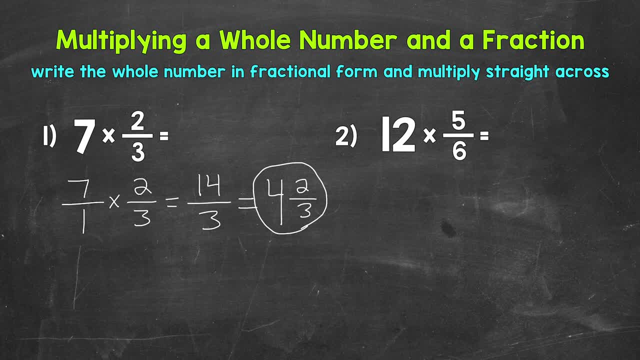 Now, just as a quick recap, as far as how we went from 14 thirds, 14 over 3, that improper fraction to the mixed number. again, we divided the numerator, so 14, and we divided by the denominator 3.. 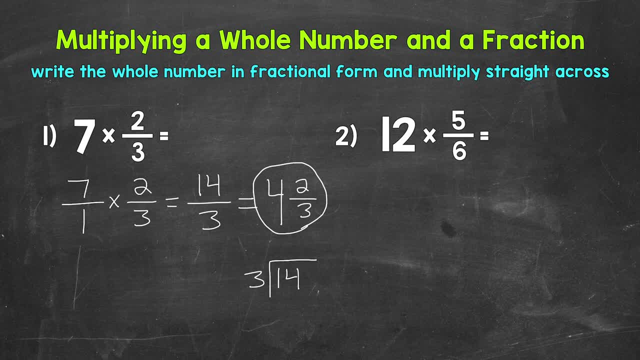 So 14 divided by 3. How many whole groups of 3 in 14?? Well, 4 whole groups. That's the whole number. portion of our mixed number 4 times 3 is 12.. Subtract 14 minus 12, gives us 2.. 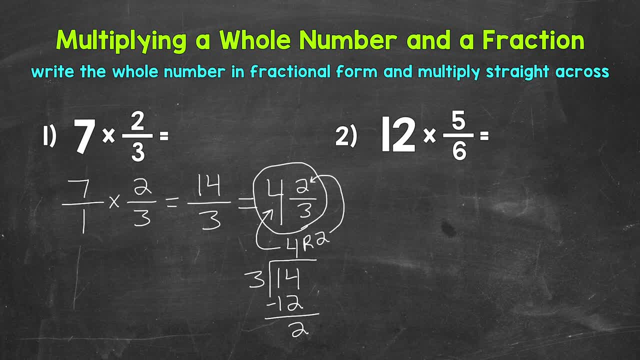 So a remainder of 2.. That's the numerator of our fractional part of the mixed number. And then we keep the denominator of 3 the same, So 4 and 2 thirds. Let's move on to number 2, where we have 12 times 5 sixths. 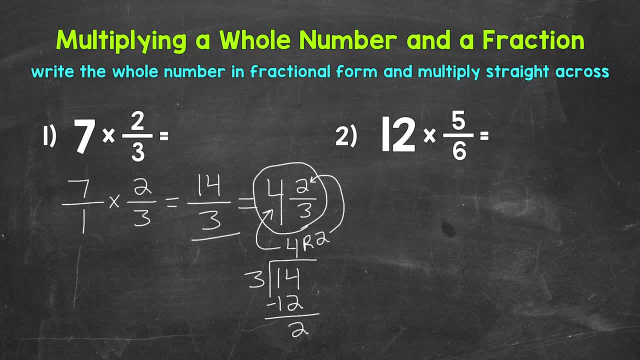 So let's rewrite 12 in fractional form by putting it over 1.. So we have 12 times 5 sixths. Now we can multiply straight across. Let's start with the numerators: 12 times 5 is 60.. 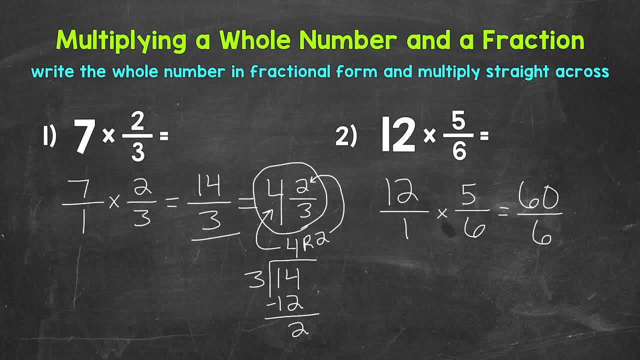 Now for the denominators: 1 times 6 is 6.. So we get 60 sixths or 60 over 6. And that's our answer. but it's an improper fraction, So let's convert it to a mixed number. 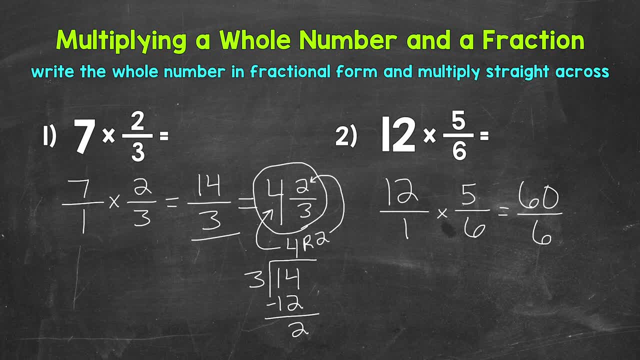 Let's divide the numerator 60 by the denominator 6.. So 60 divided by 6. How many whole groups of 6 in 60?? Well, 10.. That hits 60 exactly. We don't have a remainder.